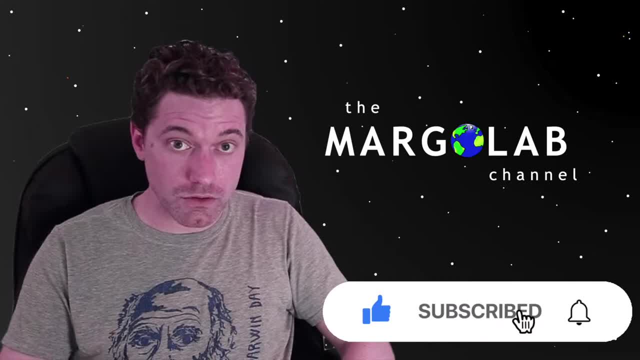 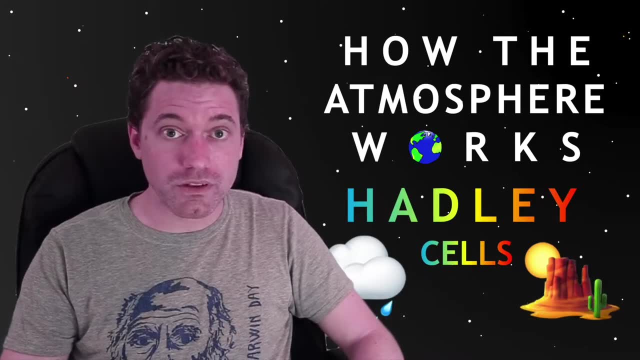 get into that. make sure you like this video and subscribe to the channel so you don't miss future videos. All right, so Hadley cells relate to, and or are responsible for, the distributions of ocean surface temperature and salinity that we learned about in how the ocean works. So we 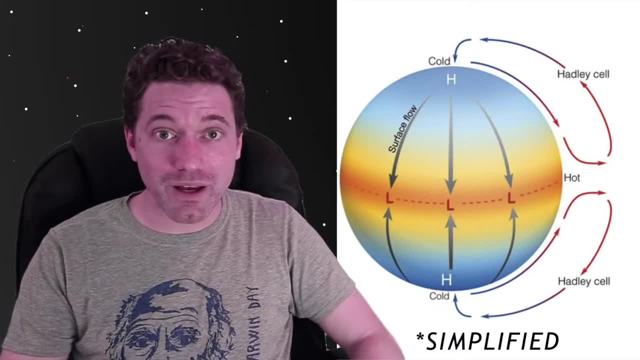 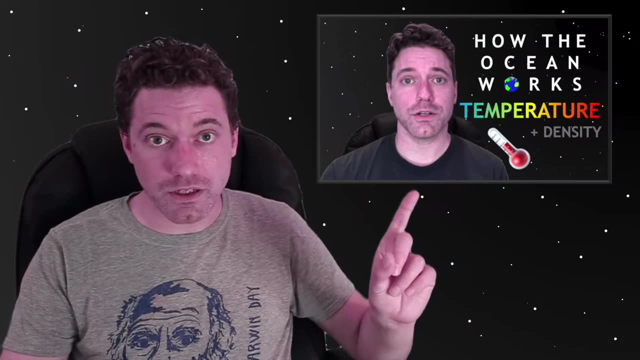 got to talk about them here. Hadley cells are driven by the fact that the equator is warm, which relates to the temperature and density of water that we talked about in this video. Personally, I like to think about gases as liquids, because for me, the movement of 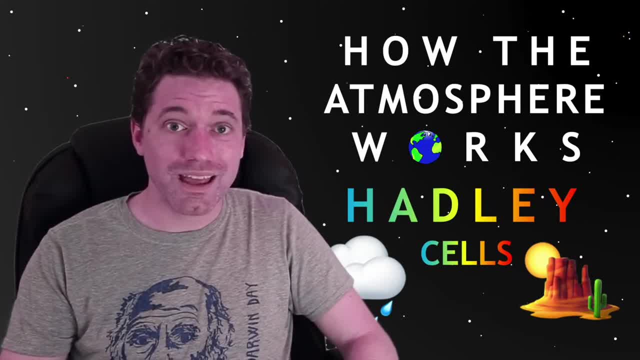 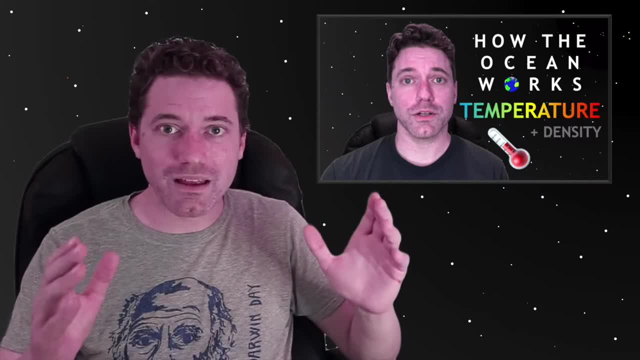 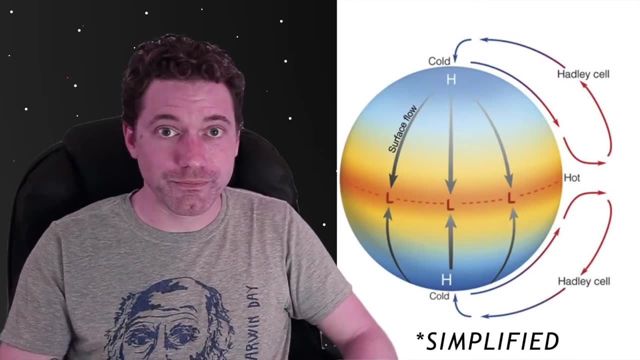 liquid is easier to visualize than the movement of gas And in many ways they behave the same. So in In the example from this video, when water is warmed, it expands, making it less dense or more buoyant, which is exactly what happens with air in the atmosphere at the equator. 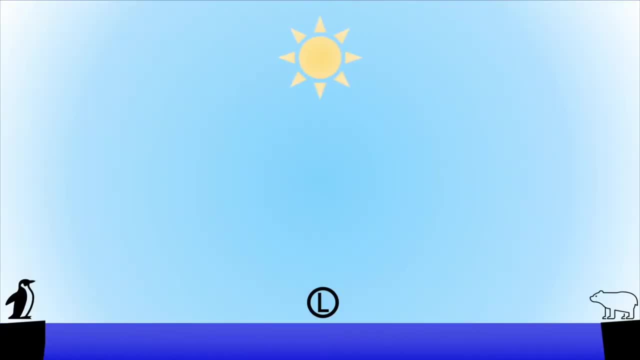 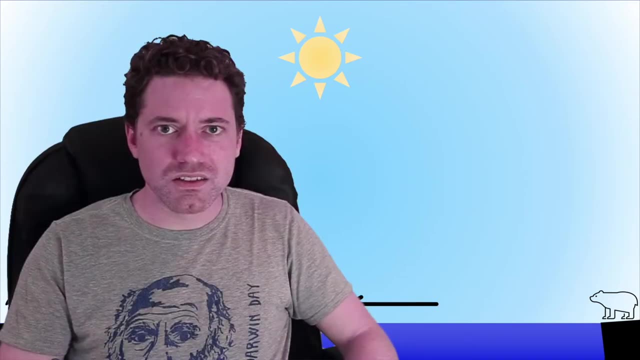 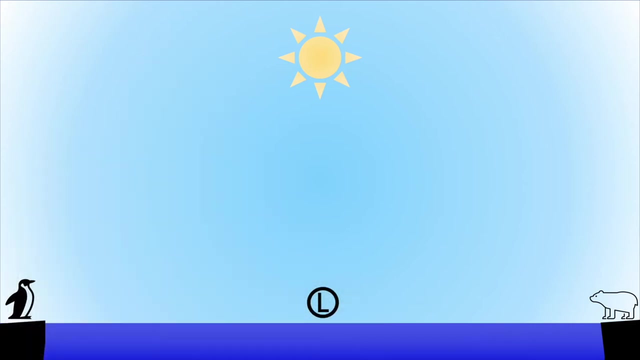 This expansion is related to there being low pressure near the equator as a result of warming, causing an equatorward flow of air along Earth's surface, just like how air flows or rushes out of a pressurized bicycle tire to the unpressurized atmosphere. 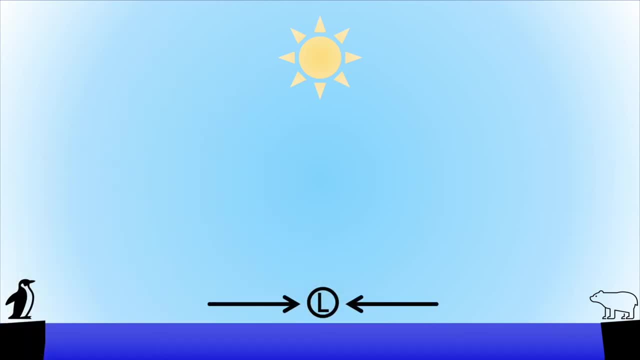 Due to the flow towards the equator, there is a convergence of air from the northern and southern hemispheres, and this converging warm, buoyant air rises up into the atmosphere. As the air rises, any moisture that it carries is wicked away to form clouds and precipitation. 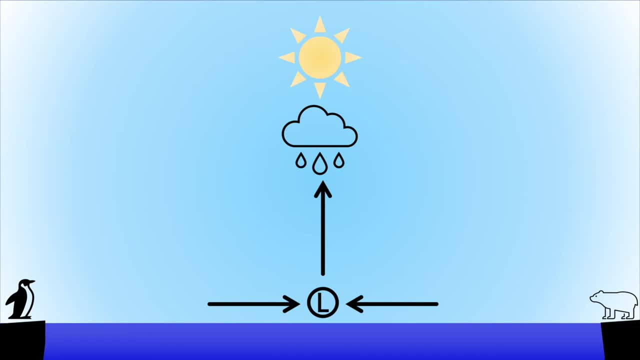 resulting in tropical rainforests and low ocean salinity due to the dilution of salty ocean water with fresh rainwater. Once this rising air has been thoroughly dried high in the atmosphere, it diverges to the north and south, making its way towards the poles. However, due to the rotation of the Earth, this poleward transport of air weakens and the dry air descends to Earth's surface around 30 degrees north and south, where we find deserts and high ocean salinity due to aridity. 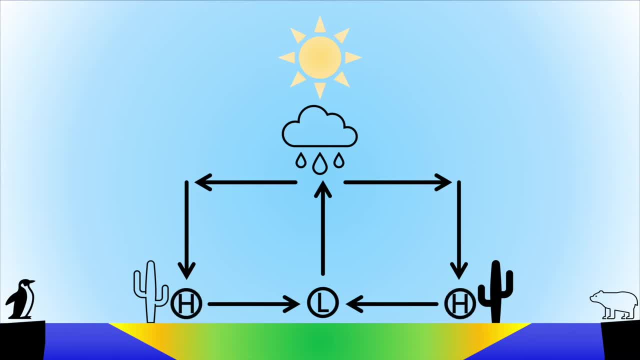 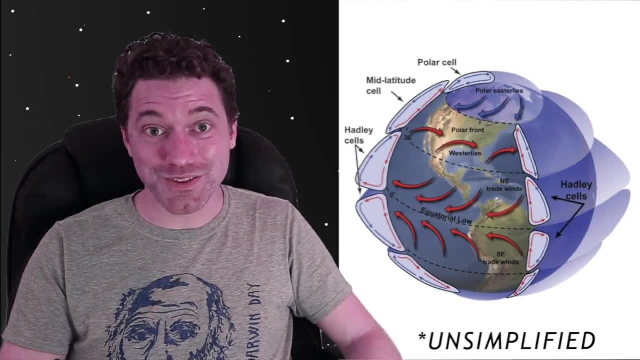 These latitudes are associated with high pressure, so this air flows back towards the low pressure at the equator and the Hadley cell circulation pattern repeats. I hope you enjoyed this video. Let me know if you'd like to learn more about how the atmosphere works and I'll see you. in the next one, Take care.